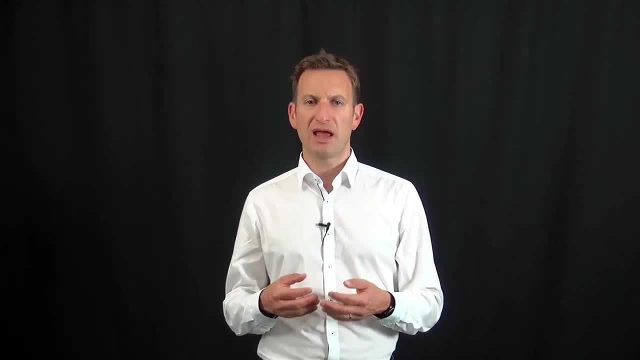 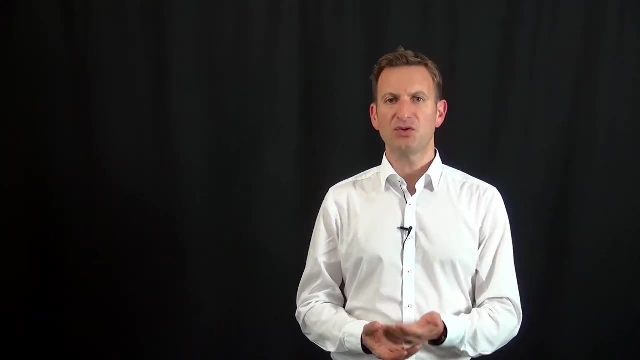 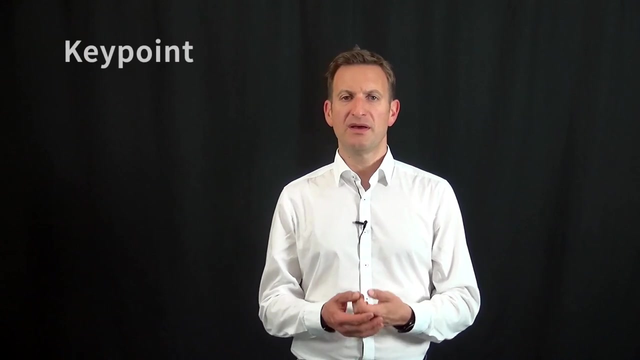 of different algorithms require features extracted from images and that the subsequent algorithms only work with those features in an image. And we have to distinguish here the computation of the key point and the computation of the descriptor vector. So how does it work? The locally distinct point, so the key point, is found using a difference of Gaussian approach. 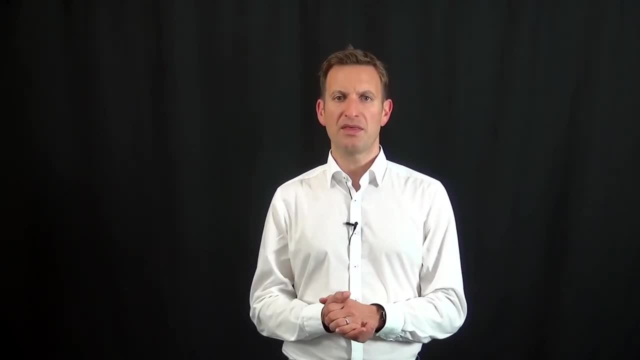 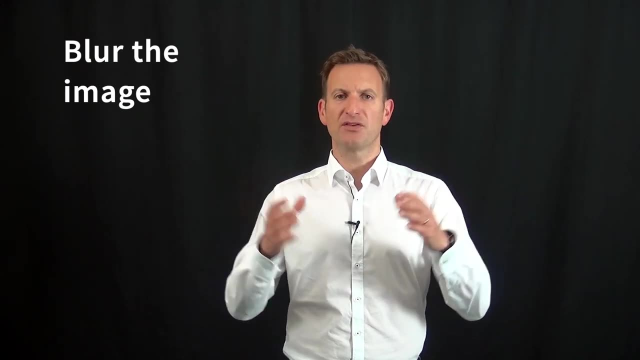 That means you take your image and you blur that image with a Gaussian blur at different magnitudes, So of an image which is slightly blurred and an image which is more blurred, and so on and so forth, And then you subtract those images from each other. 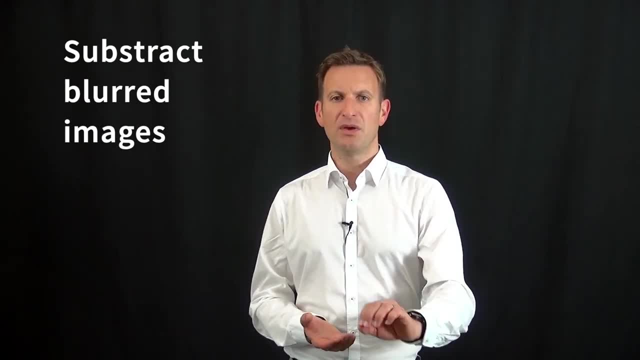 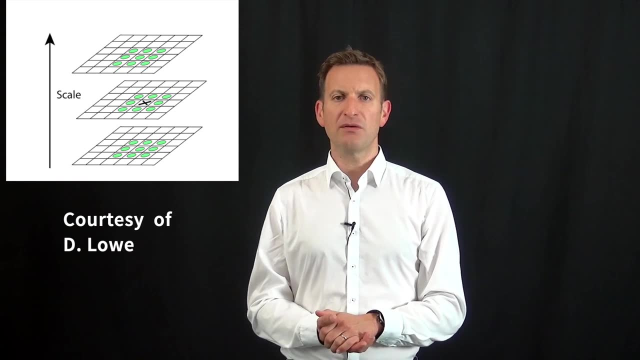 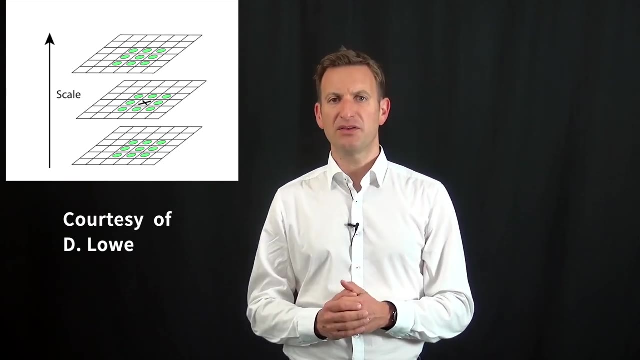 So you basically get a difference of images with different levels of Gaussian blur And then you stack those difference images On top of each other And you're basically looking for extreme points, So points where all the neighbors in the XY image space, as well as in the space of different 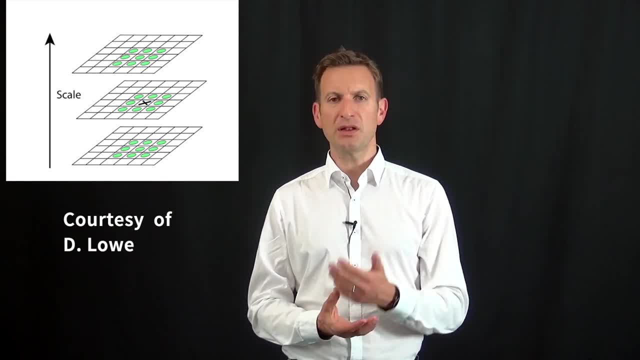 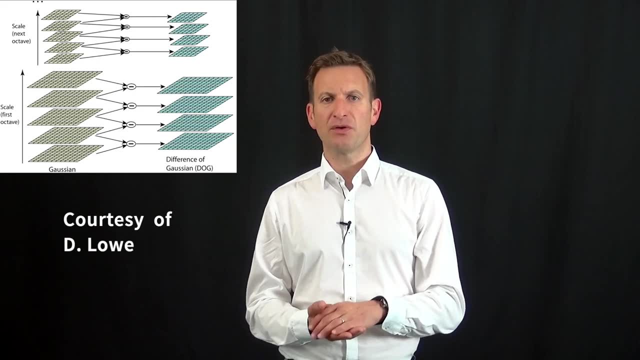 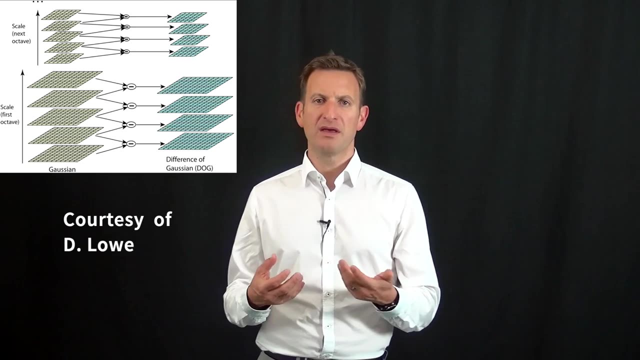 levels of smoothing which are locally distinct, which stand out And those are your key points. You typically don't do that only for one image resolution. You also perform this of an image pyramid. That means images which are differently scaled in size in order to find key points. that also. 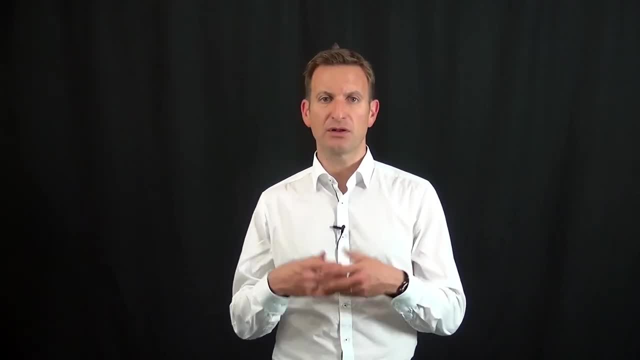 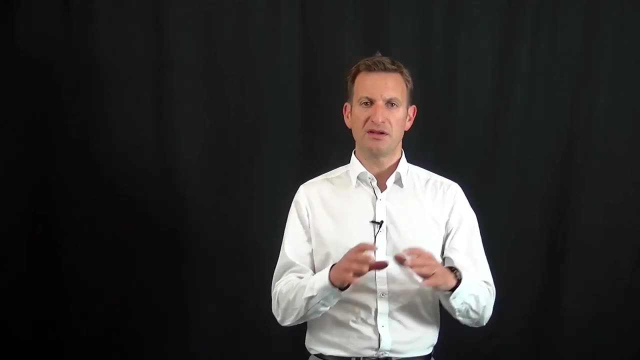 are distinct With respect to scale changes. So if you're closer to an object, you will still find the same key points as if you're further away. So this is about the key point. The next step is to compute the descriptor vector. 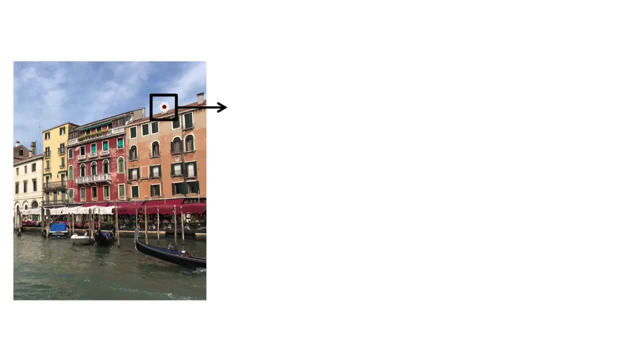 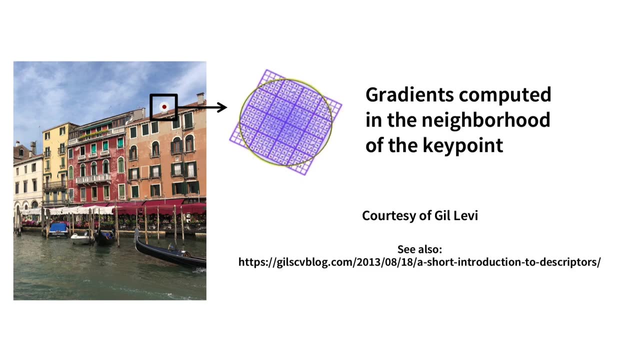 You do that by looking into the local neighborhood of the key point that you find, And what you're doing is you're basically taking the local neighborhood and breaking it down in kind of small areas and compute the gradients in these small areas, Use gradients. 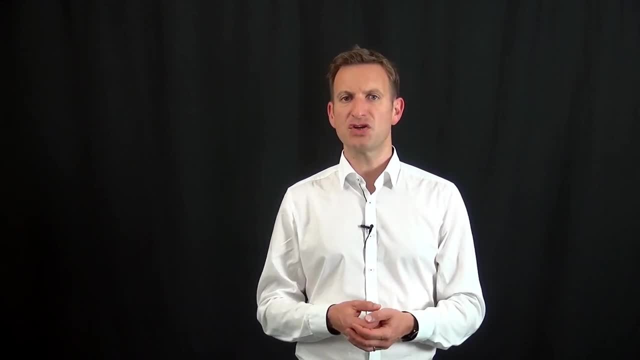 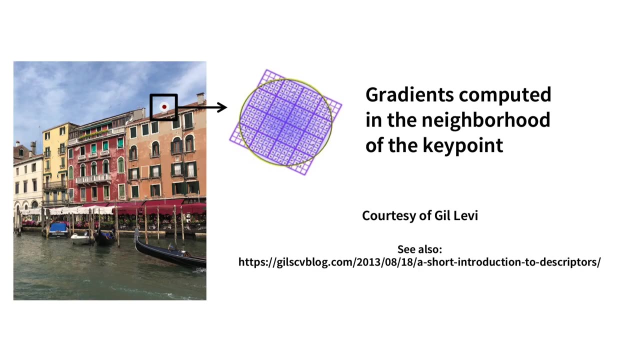 Because those gradients are typically rather robust with respect to illumination changes, Also with certain viewpoint changes. So what you do? you basically compute all those gradients and then collect gradients in local regions into histograms. So how often do certain gradients occur? What's their magnitude? 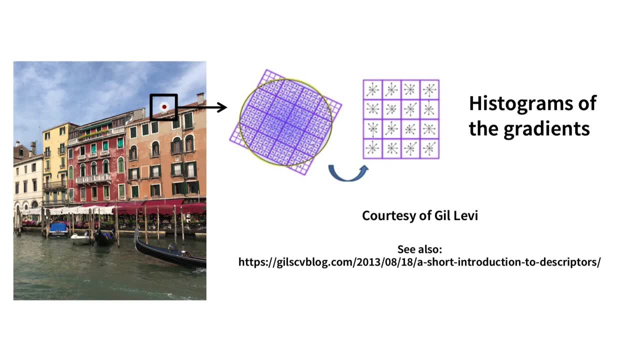 You just turn that into histograms for small local regions And in the end, around the key point in a four by four region, You compute histograms. So four times four, sixteen histograms. Every histogram is discretized in a 45 degree orientation. 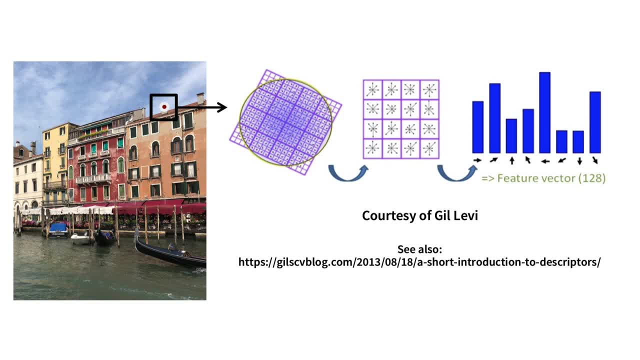 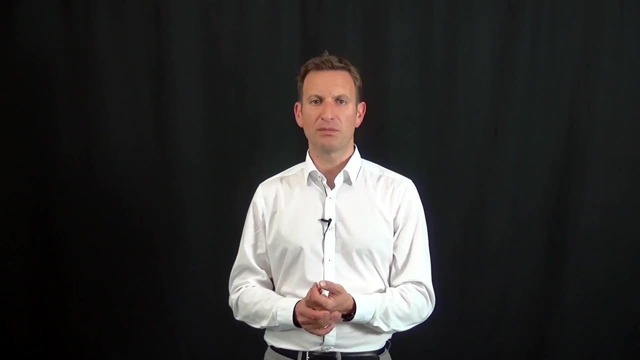 That means it has eight bins, And this gives you 128 values. You're basically just concatenating these 128 values and this gives you your descriptor vector, And this is kind of the SIFT descriptor that we are using in order to describe the local. 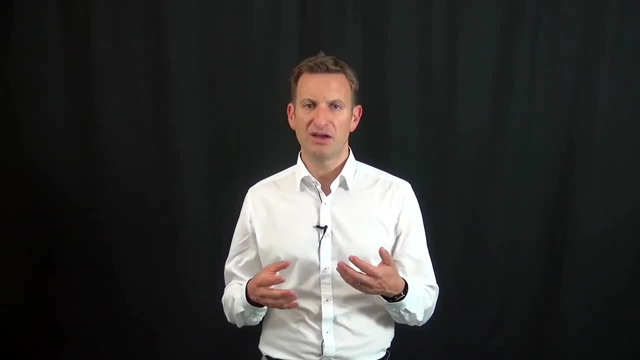 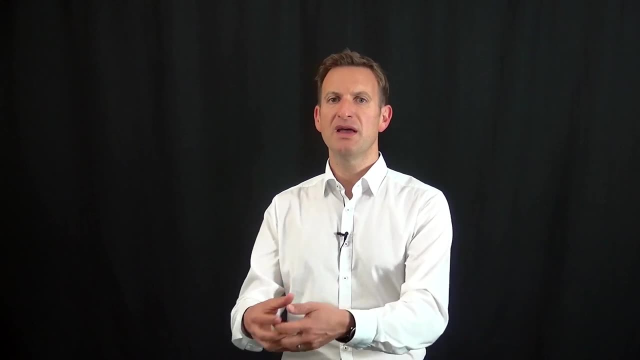 key point. I hope that gave you an idea what a SIFT feature is When we refer to it as a way for computing the key points, using the difference of Gaussian approach And then taking the gradients in the local neighborhood into account in order to compute. 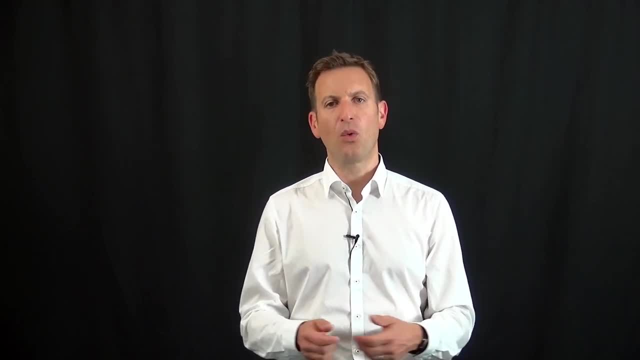 a descriptor vector that can be used to describe or identify the key point. I hope that was useful. Thank you very much for your attention.